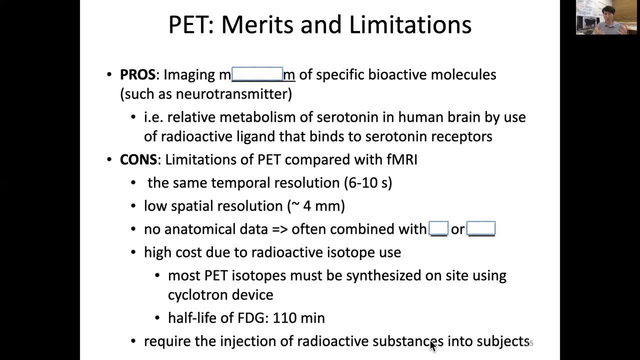 So remember, for example, our institute has a micropen but we don't have a cyclotron. In that case we have a little limited use of micropen. because in the local hospital there are cyclotron, We actually order it. 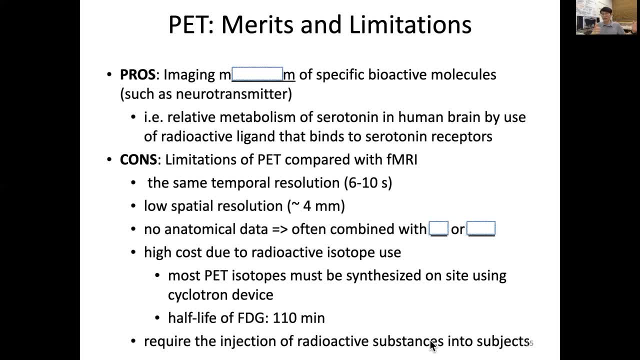 There's no cyclotron, There's a quick service delivering it within several tens of minutes. then we have only limited time interval to image for run the PET, So that is a kind of limitation, But however it gives a great metabolic information. 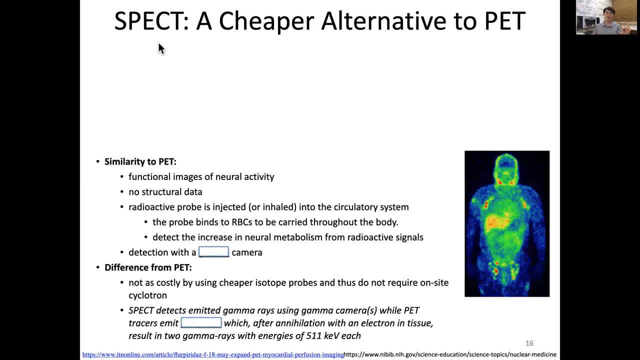 So in comparison with the PET, I want to go back to SPECT because it's a cheaper alternative to PET And in the United States alone almost 75% of nuclear medicine imaging is done by SPECT, not the PET, because PET's more expensive. 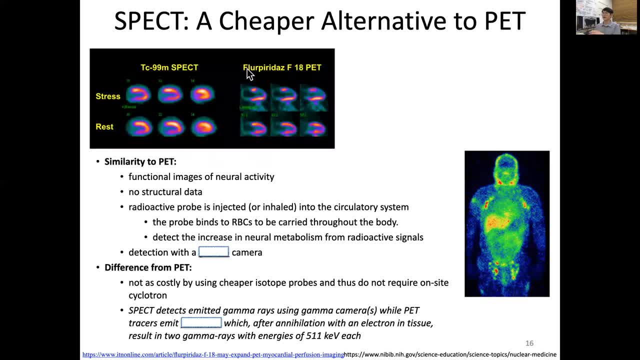 So SPECT- I'll give you one example of heart imaging under stress and rest condition and Technetium 99 base of SPECT and F18 base of PET. So this is the PET, This is the PET And this is the PET. 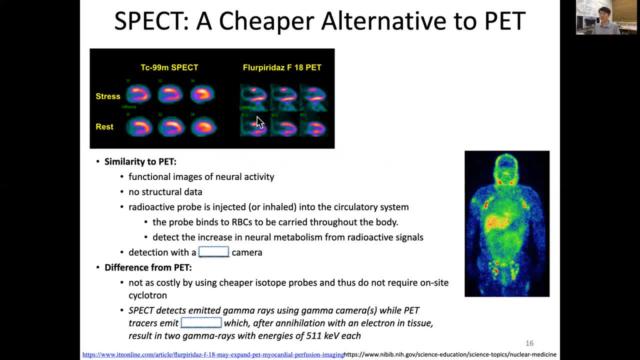 Now in the individual population, we have said two times in one click. we have a very little ignorance of the principles behind the PET. These are things that quote unquote as factors of physical damage And this alone is already happening. This is a big part of our health, ever since we started the- whatever they call- glac forge. 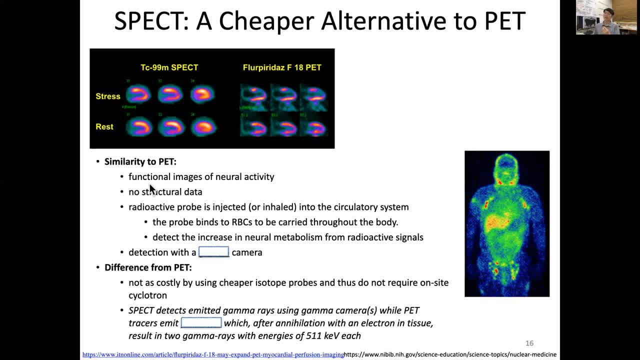 from radioactive signals, And both, not both. SPECT uses a detector with a gamma camera. So here I have a little bit of a table comparison. SPECT emits gamma radiation by a path that radioisotope emits positive force and then that converts. 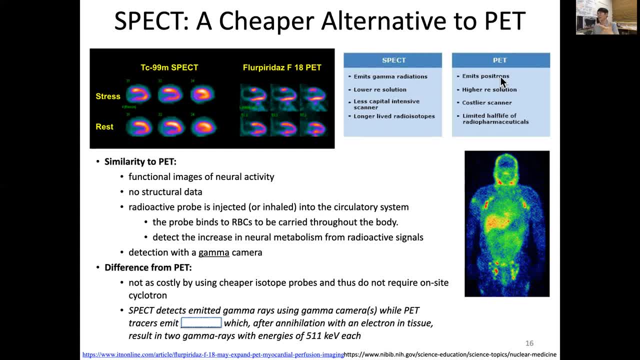 into the opposing pair of a gamma rays And, in terms of resolution, PET has a little higher resolution and SPECT uses long-leaved radioisotope which can be cheaply manufactured or made, while PET case we have a limited half-life of.